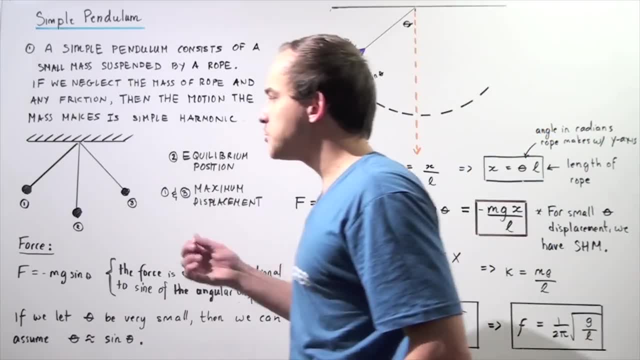 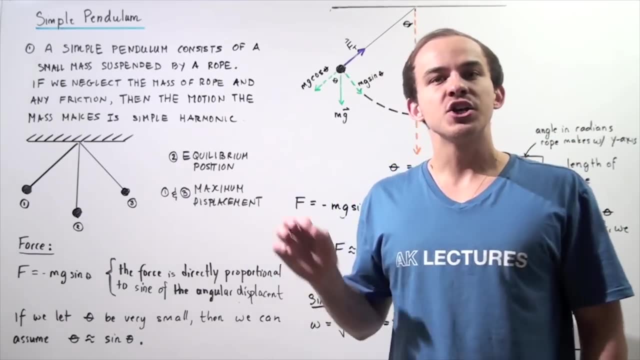 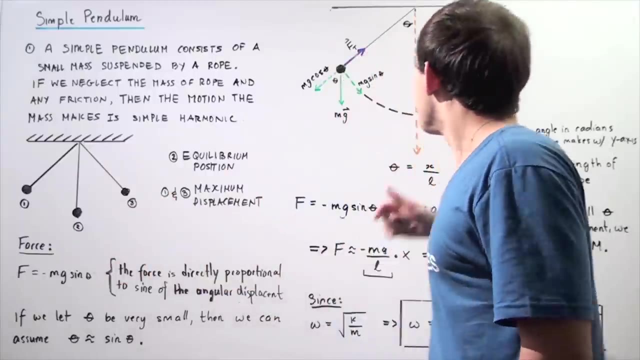 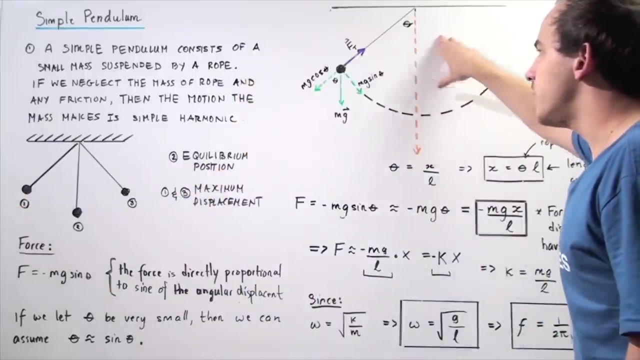 all the forces that are acting on our object at position one, and then we want to use those forces to determine the actual force that creates our oscillating motion, that allows our object to swing back and forth. so let's look at the following diagram: and we're only looking at position one. so at position one we 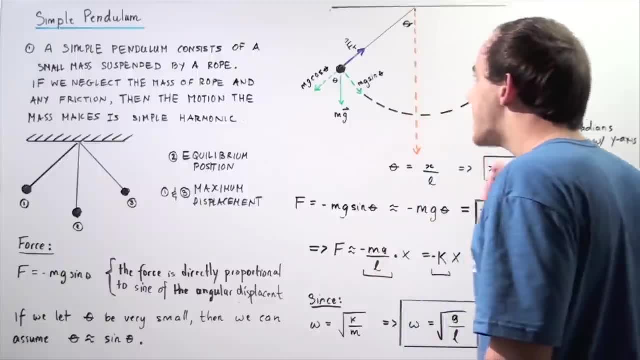 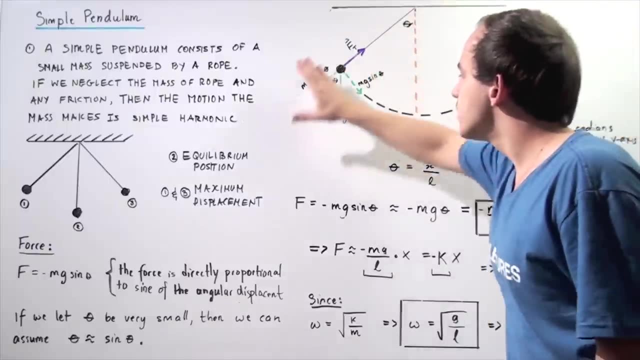 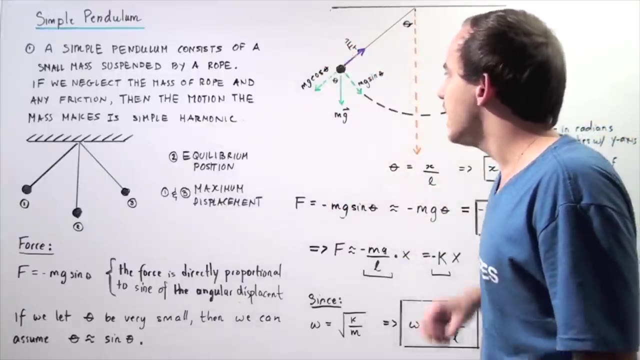 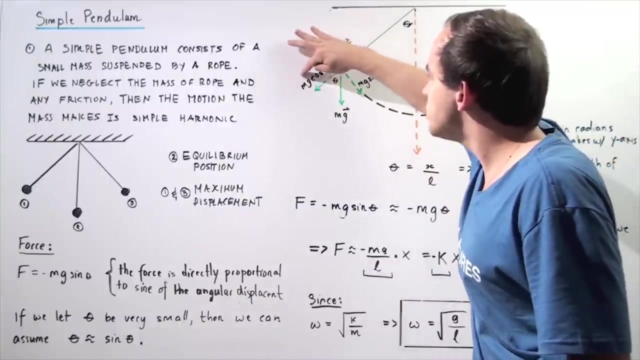 have two forces acting on the object. we have the tension in the chord that points along the chord in this direction, and we also have the force of gravity that's pulling downward on our mass. so this force of gravity has two component forces acting on our mass. we have this component force, M times, G times, cosine. 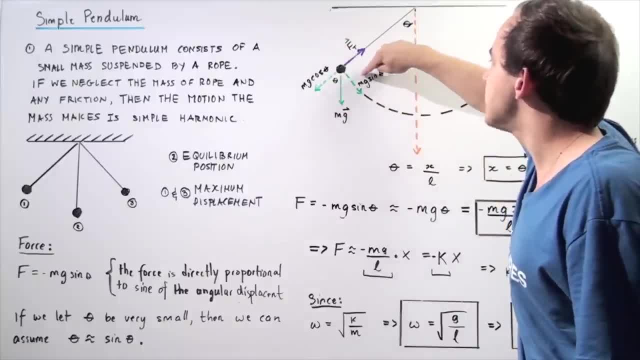 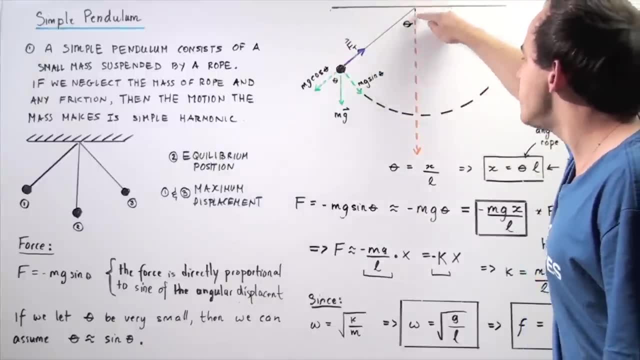 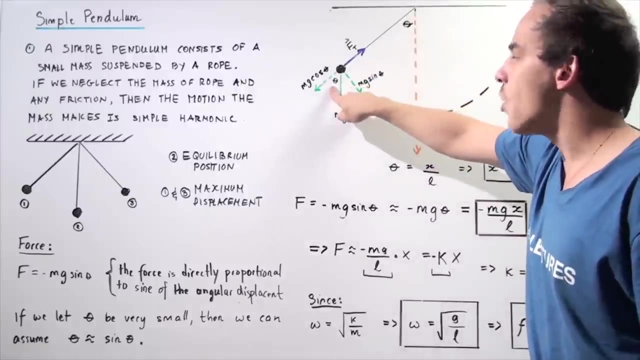 Theta and this component force, which is M times G times theta. Notice, the theta is simply the angle that the rope makes with our imaginary y-axis shown in orange. So if this angle is theta, this angle is also theta, And that means we get mg cosine. 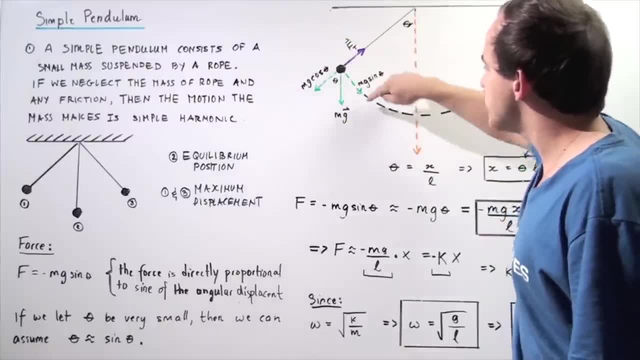 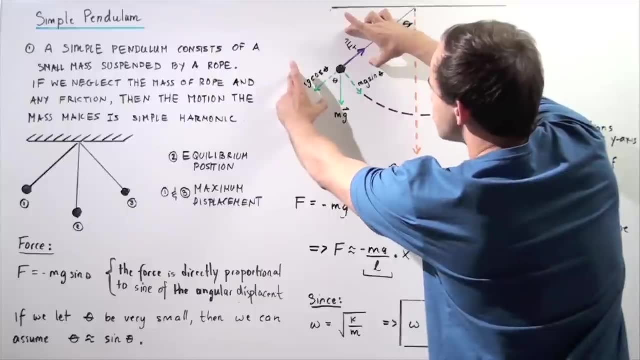 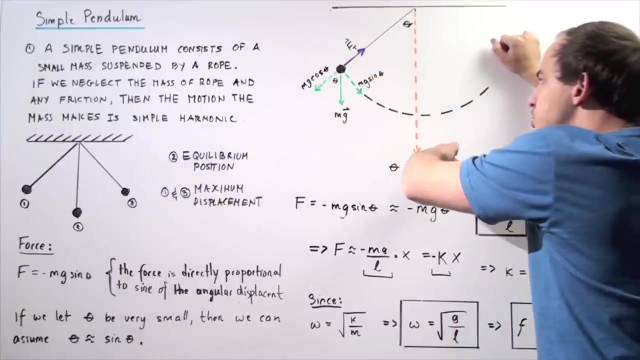 theta for this vector and mg sine theta for this vector. Now notice: there is no motion along this axis. So that means these two forces are equal, but we do have a net force acting on the mass that points in this direction, And that net force is the result of mg sine theta. So this is the 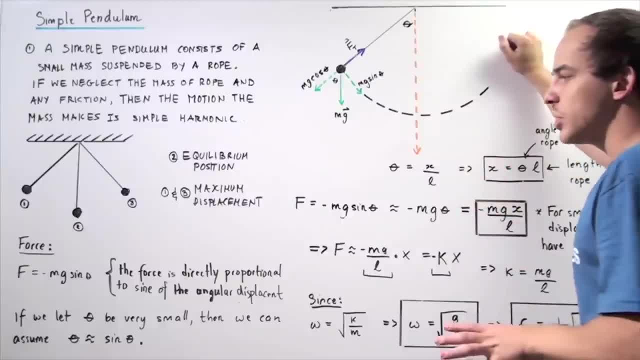 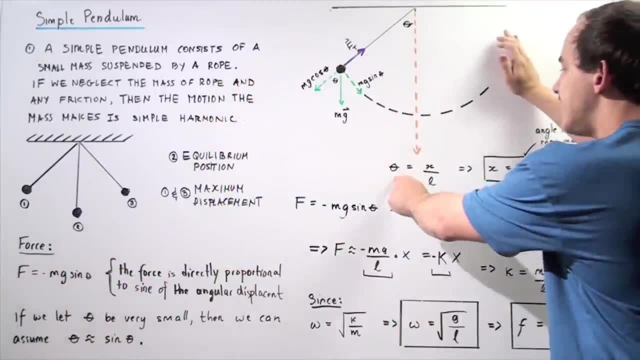 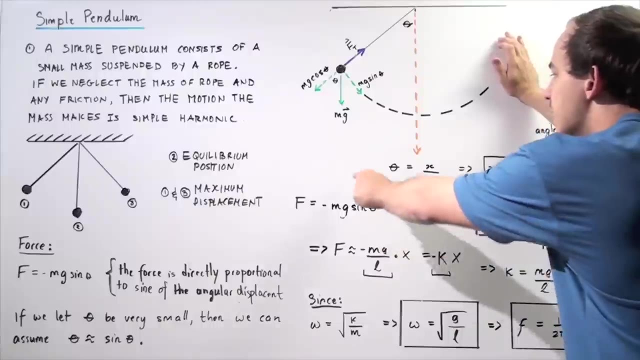 force that creates our oscillating motion. So f is equal to negative mg sine theta. Now, what exactly is theta, Where theta is also known as the angle? So theta is the angular displacement of our object, And recall that the angular displacement of the 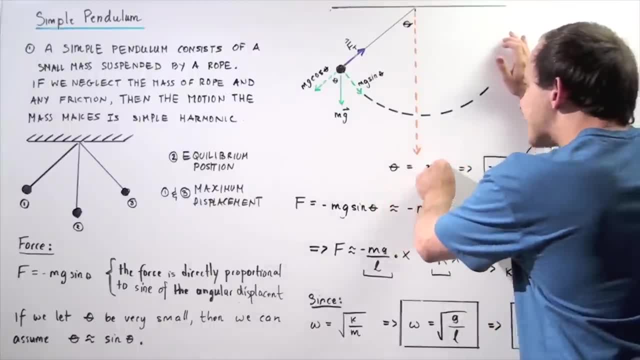 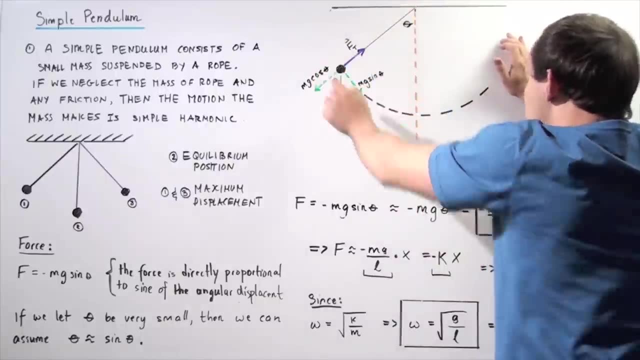 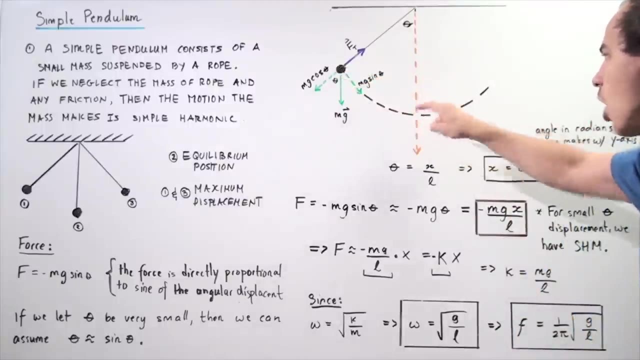 object given in radians is equal to x, our displacement along the following arc, divided by l, which is the length of our rope. So if we rearrange this equation, we see that our displacement of the object along this arc is equal to our angle in radians that the rope makes with respect to our 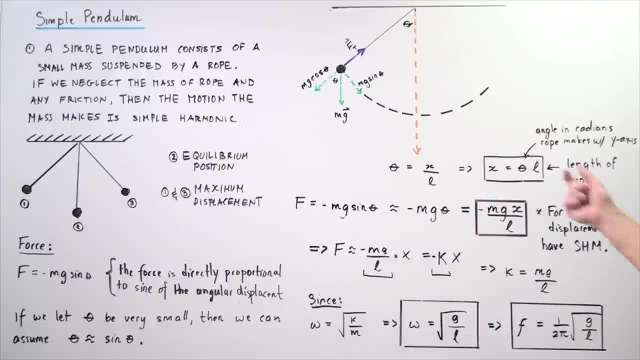 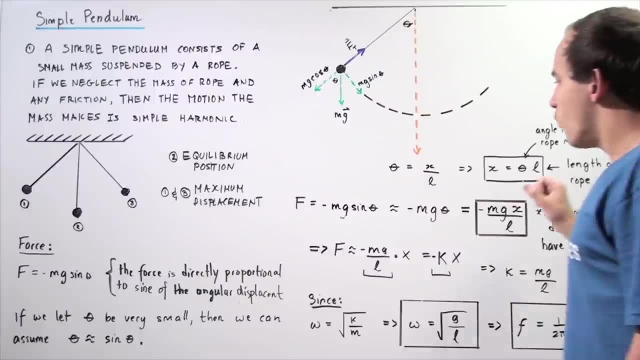 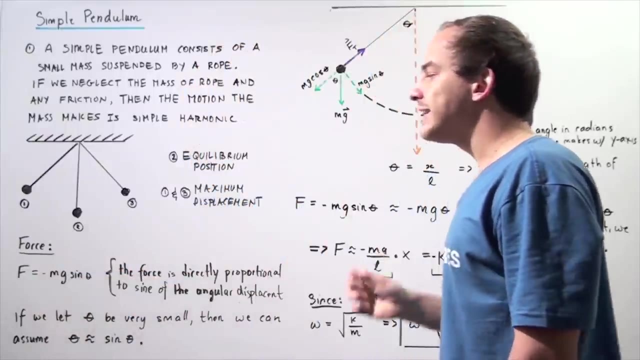 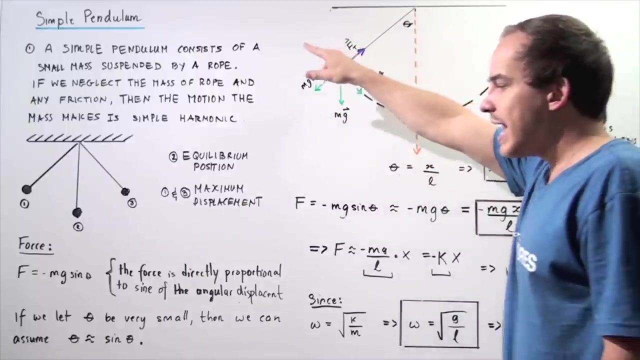 vertical axis x is also known as our angular displacement, multiplied by l, our length of the rope, given in meters. So before we continue with this step, let's go back to this formula. So this formula tells us that the force acting on our object, that's propelling the object to swing back and forth, is: 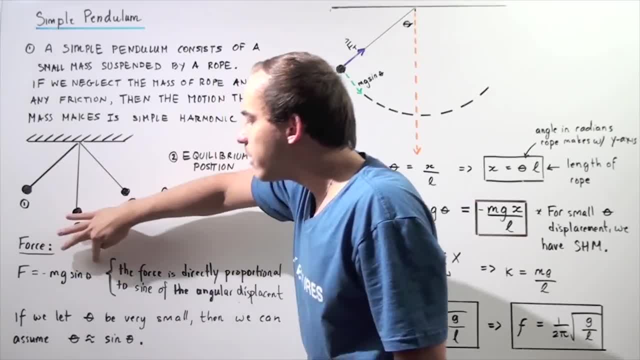 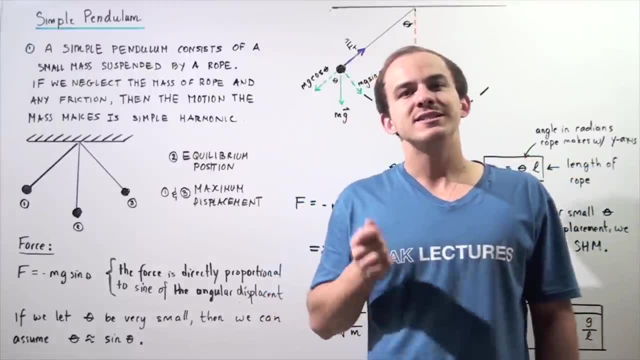 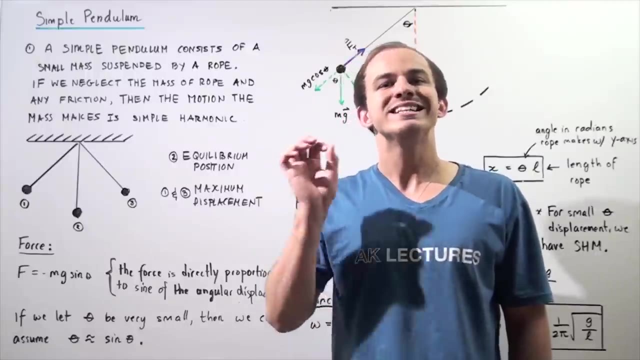 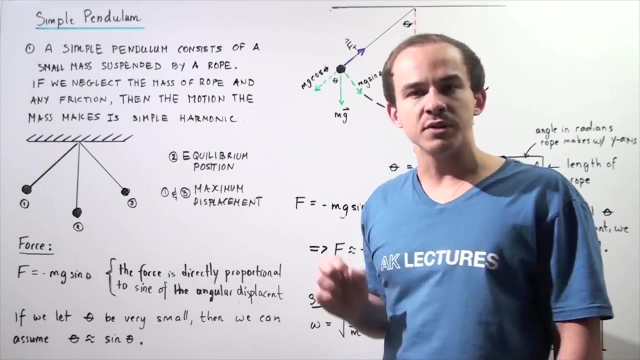 directly proportional to the sine of the angular displacement. Now recall, by definition, whenever an object is undergoing simple harmonic motion, the force that object feels is directly proportional to the displacement. And in this case the force is directly proportional to the sine of that displacement. So that means our swinging pendulum is not really. 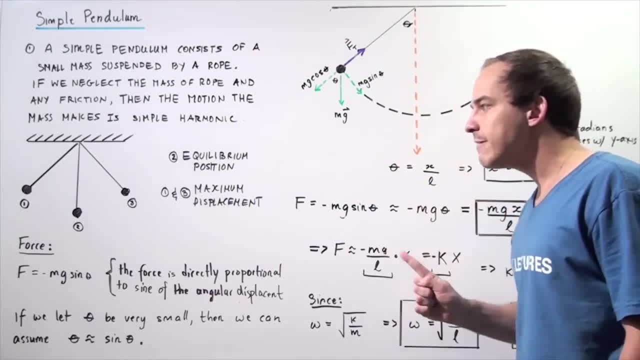 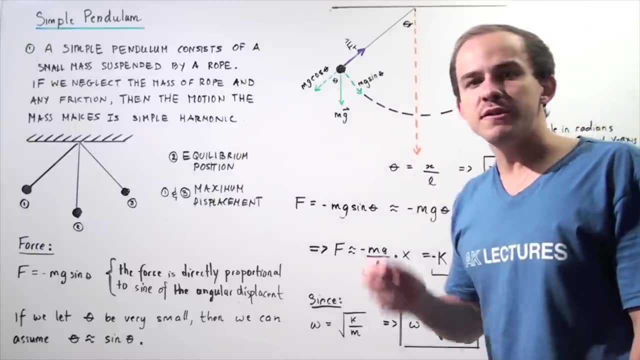 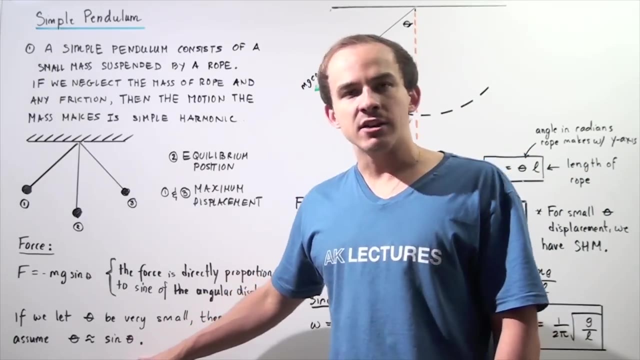 undergoing simple, harmonic motion. However, notice that if we allow our pendulum to swing back and forth, our angle that the rope makes, with respect to the vertical axis, to be very small, then that angle is approximately equal to the sine of that angle. In other words, when the angle is small, we have the 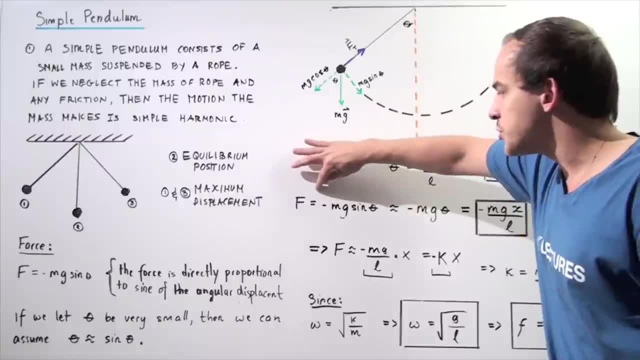 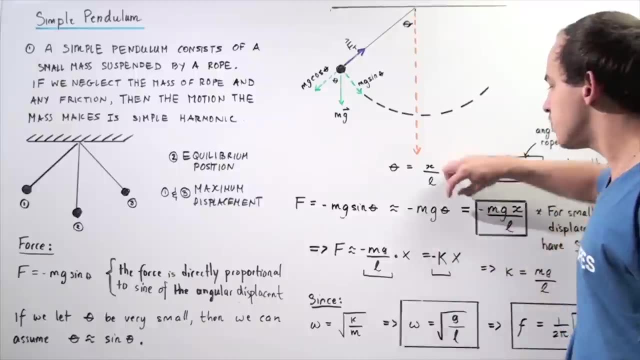 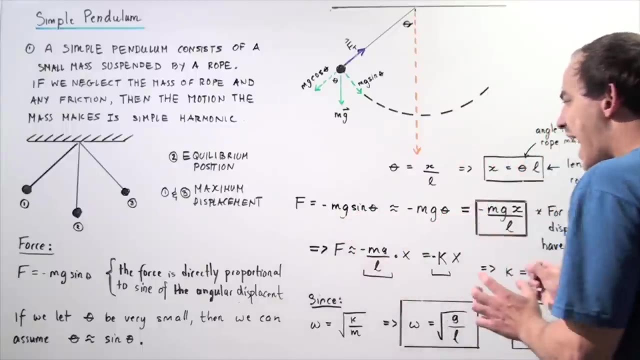 following approximation. So that means force which is equal to negative mg. sine of the angle theta is approximately equal to negative mg of the angle theta, Because when the angles are small these two quantities are approximately the same. And now we have the following equation: Force is: 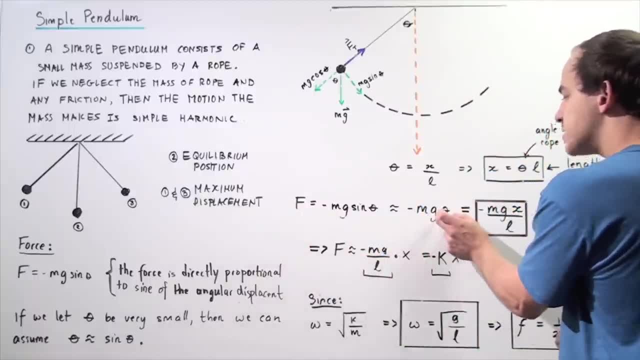 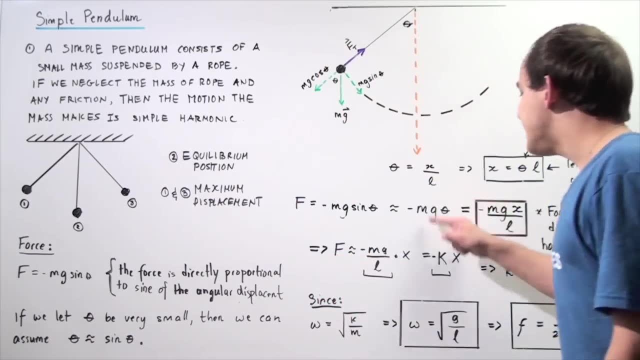 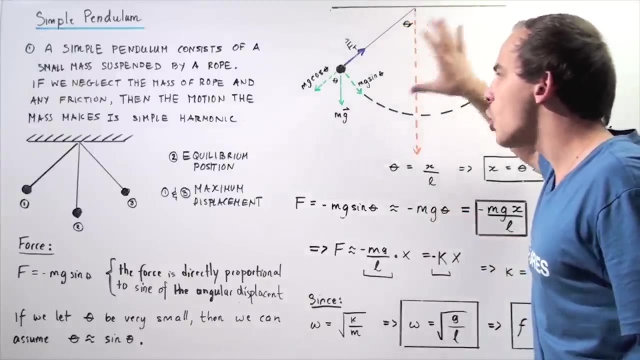 approximately equal to negative mg of the angle displacement, and we see that our force is now directly proportional to our angle displacement. So that means when the angle is small is assumed to be small, when there is no fraction and when the mass of our chord is assumed to be zero. 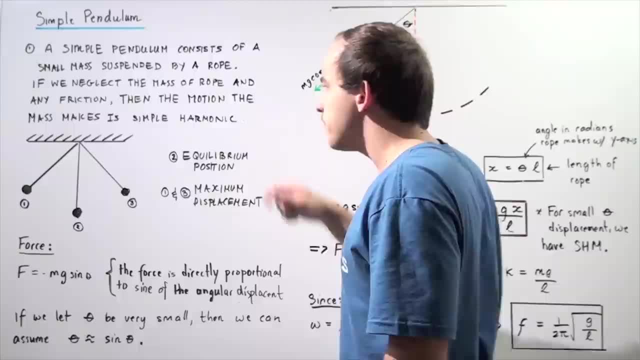 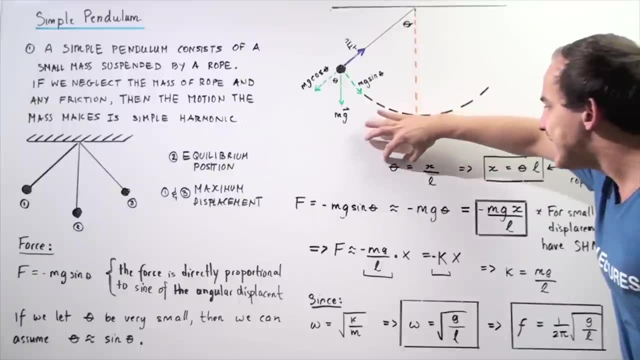 then the angle is small. So that means when the angle is small is assumed to be zero. when the, then our object, our simple swinging pendulum, is undergoing simple harmonic motion. Now notice from this result, because our angular displacement is equal to x divided by L.